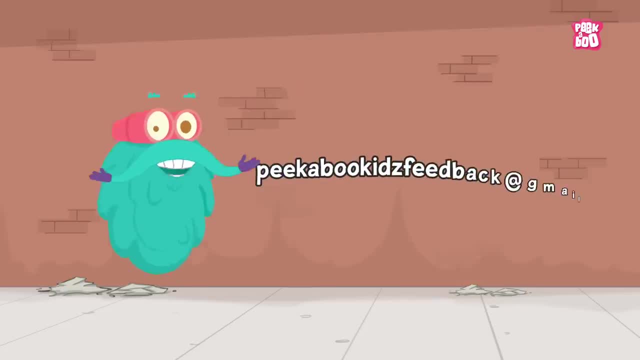 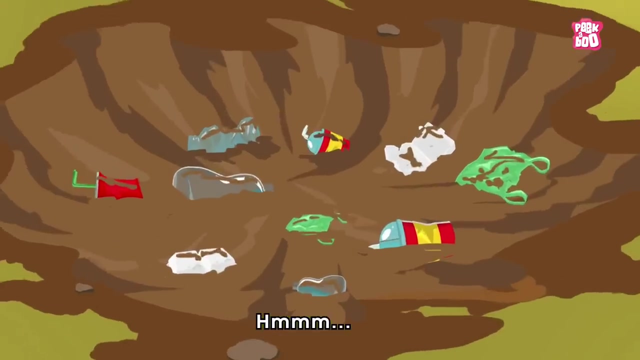 at our email id: peekabookidsfeedback at gmailcom. Similarly, you can also visit our Instagram and Facebook page and continue to engage with us. We are looking forward to hearing from you. Oh look, little kitty, it's plastic. Oh no. 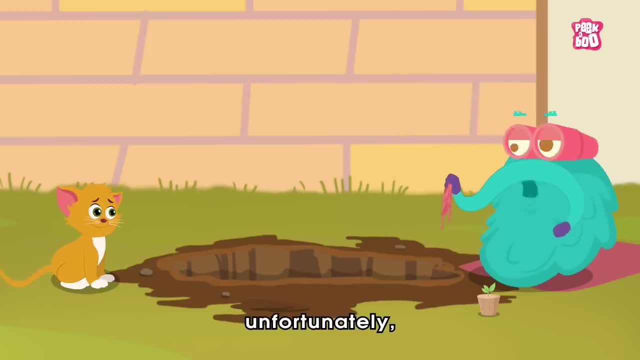 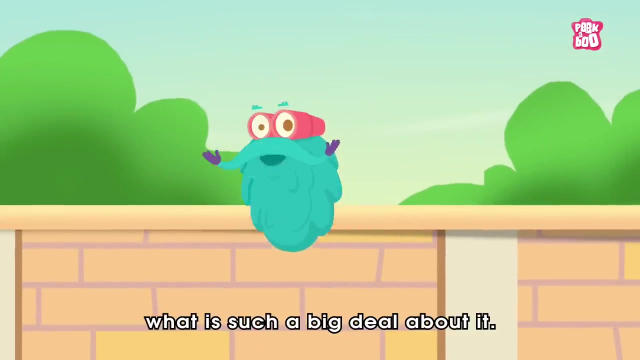 Oh yes, little kitty. unfortunately, this has become a very familiar sight, as the world is getting engulfed in plastic waste. Hey friends, I am sure you guys must be wondering what is such a big deal about it. Well, you won't believe, but plastic pollution has become one of the most urgent environmental issues we are facing presently. 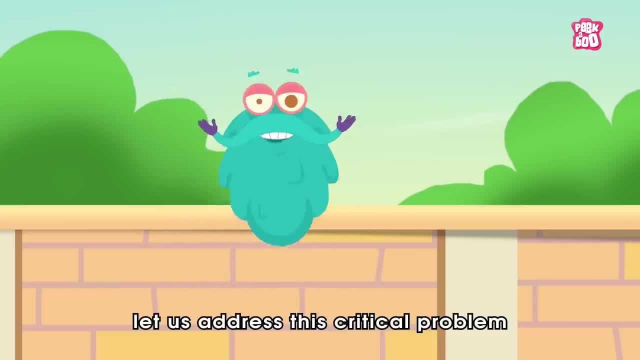 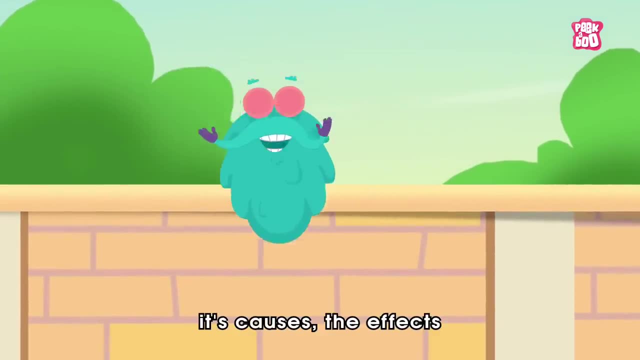 So in today's episode we are going to talk about plastic pollution. So in today's episode we are going to talk about plastic pollution. In this episode, let us address this critical problem and learn what is plastic pollution, its causes, the effects, the effect on us. 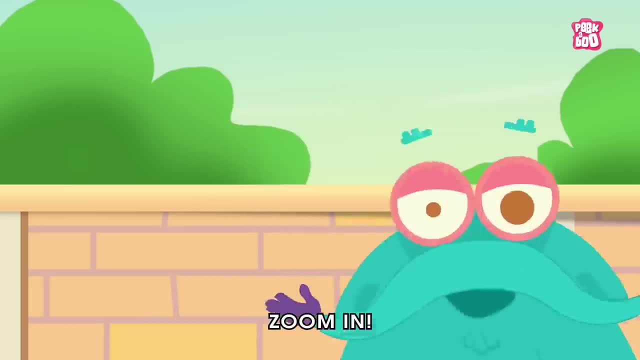 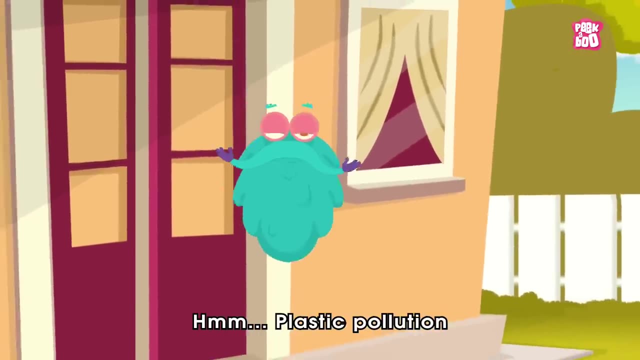 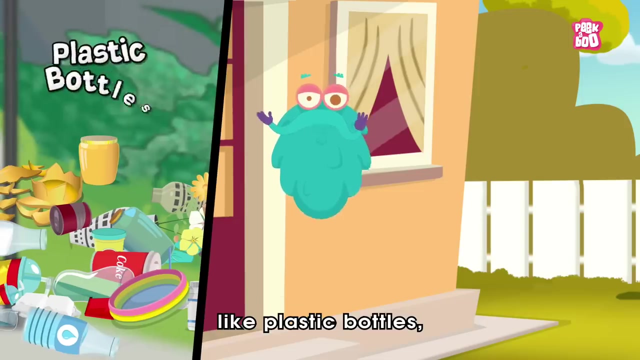 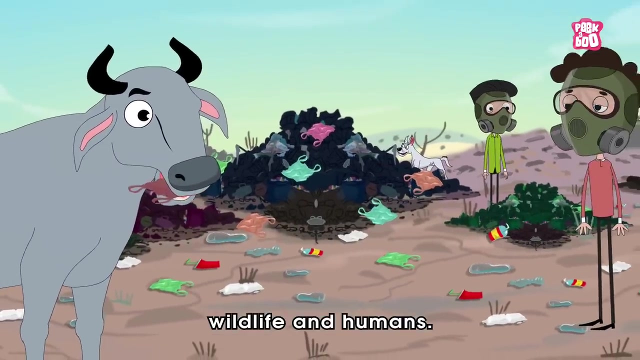 and what we can do to deal with it. Zoom in. So what is plastic pollution? Plastic pollution is the accumulation of plastic objects and particles- like plastic bottles, bags and microbeads- in the earth's environment that adversely affects wildlife and humans. 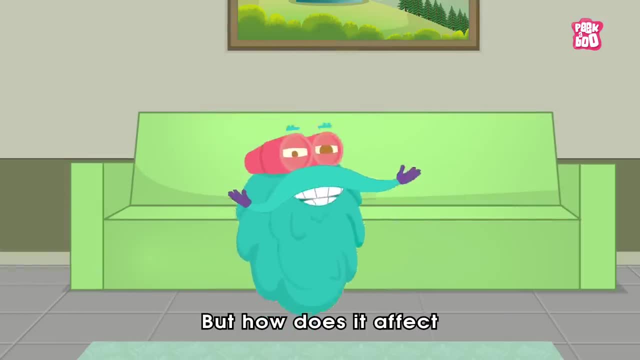 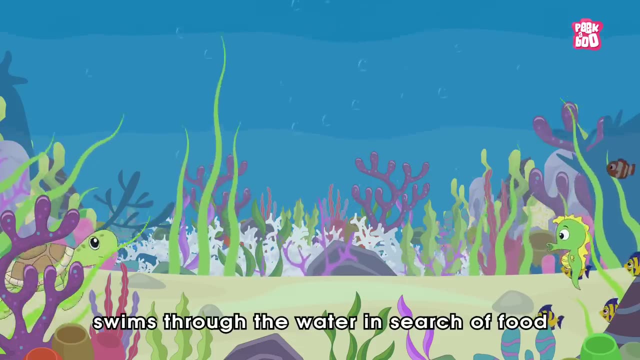 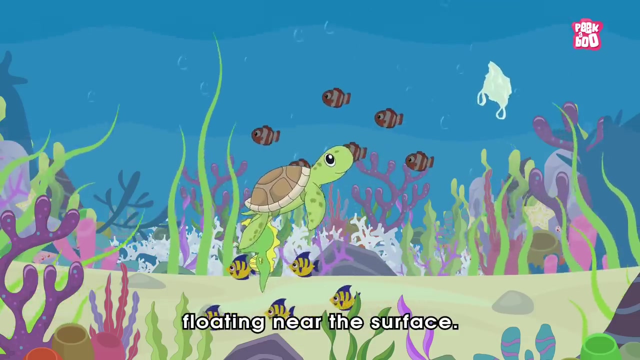 I know what you guys are thinking, But how does it affect the lives of humans and animals? Well, imagine: a sea turtle swims through the water in search of food and finds a white blob floating near the surface. Yummy, it thinks a jellyfish and eats the item. 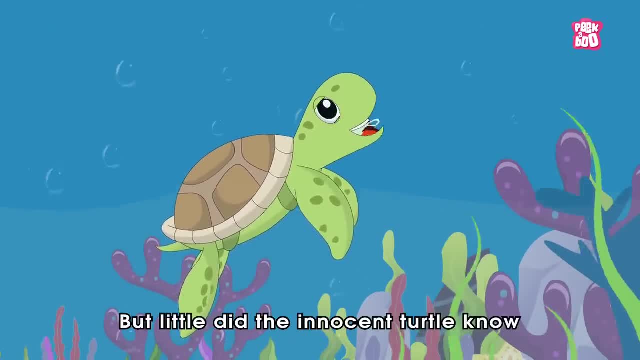 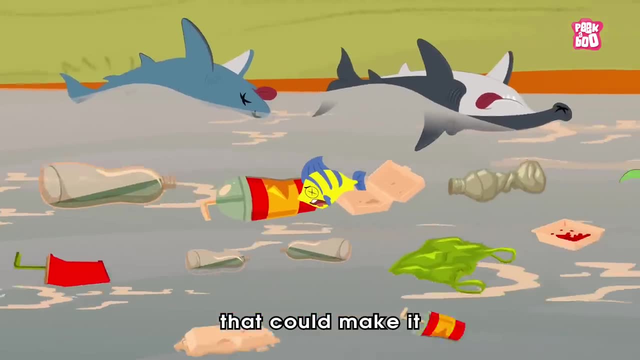 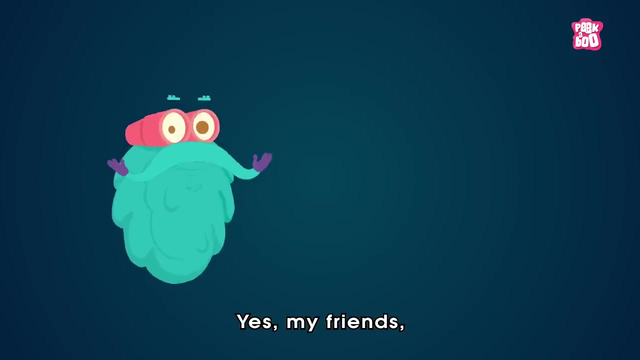 But little did the innocent turtle know that the floating blob isn't a jellyfish but a plastic bag that could make it and many other aquatic animals very sick. Yes, my friends, just like that. millions of animals are killed by plastic. 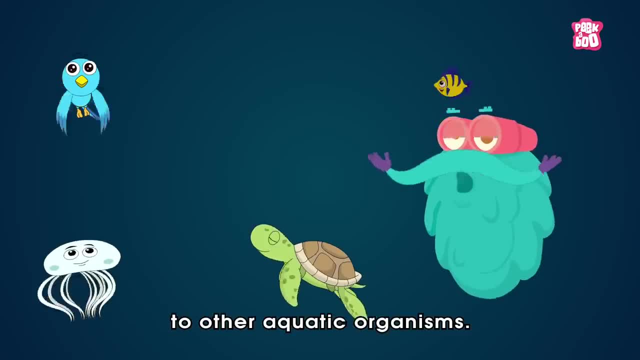 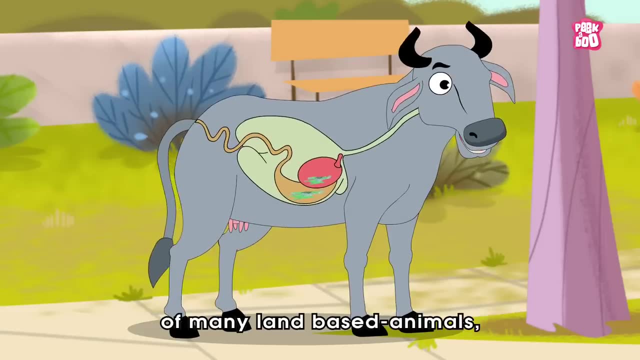 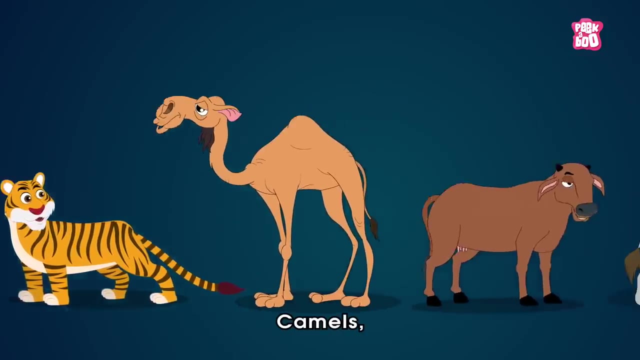 every year, from birds to fish to other aquatic organisms. Not only that, plastic has been found in the stomach of many land-based animals, including elephants, zebras, tigers, camels, cattle and other large mammals, in some cases causing death. 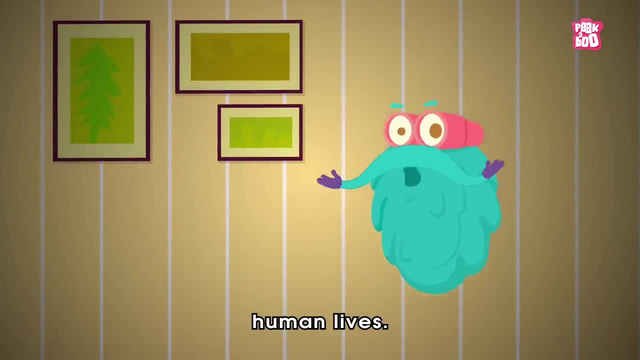 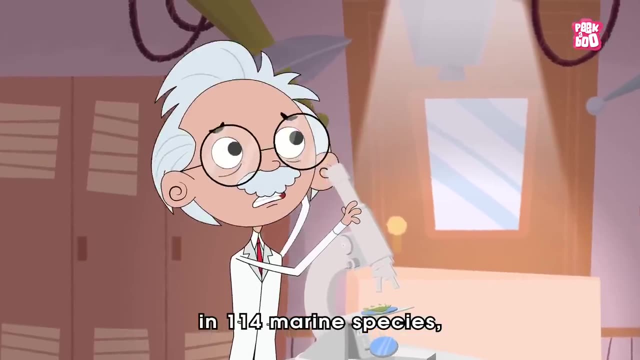 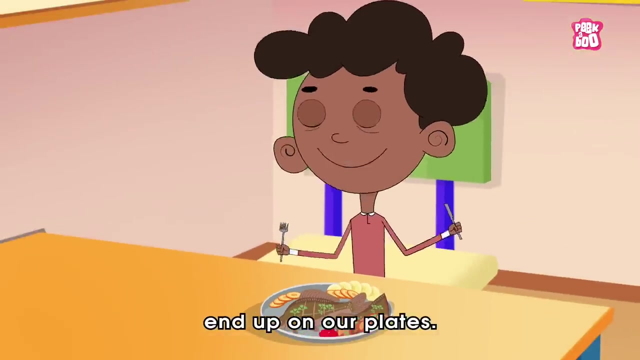 And all these factors somehow impact human lives. Yes, Scientists have found micro-plastics in 114 marine species, and almost one-third of these end up on our plates. Also, they have been found in a majority of the world's tap water. 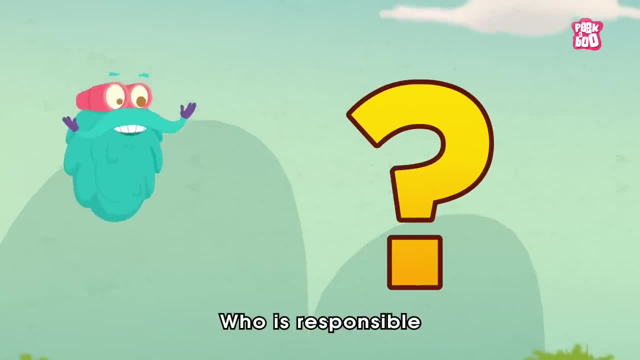 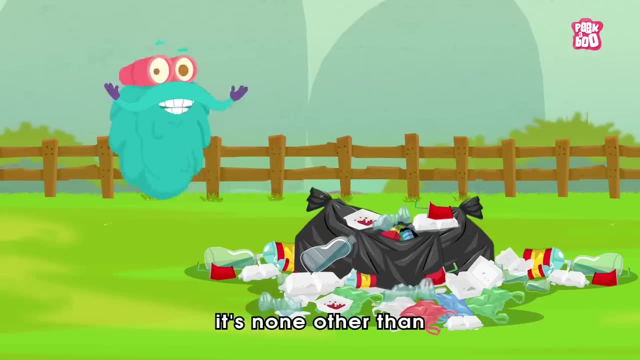 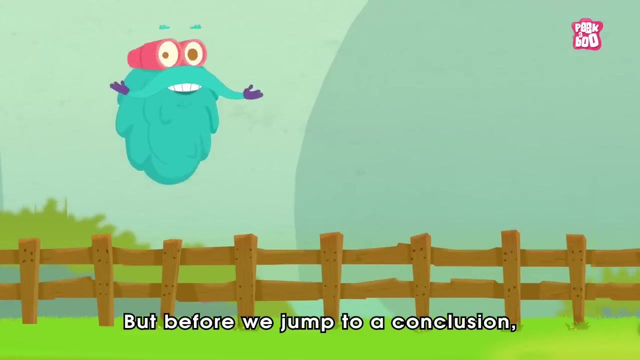 But the critical question is: who is responsible for all this plastic mess around us? Well, unfortunately, it's none other than humans themselves. But before we jump to a conclusion, we need to understand that not all plastic is terrible, as they are handy. 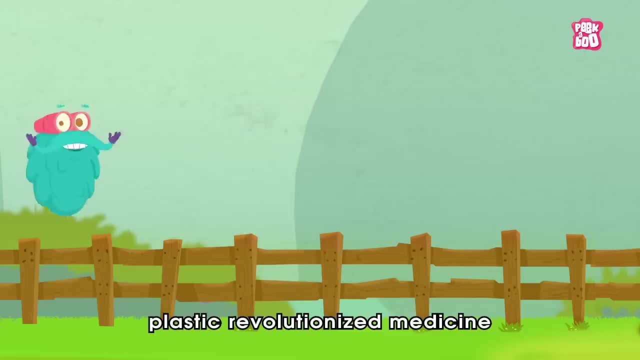 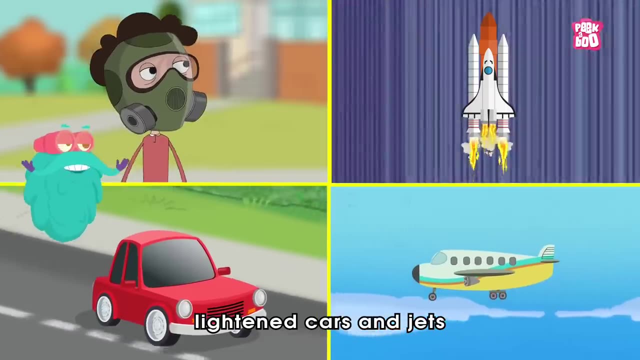 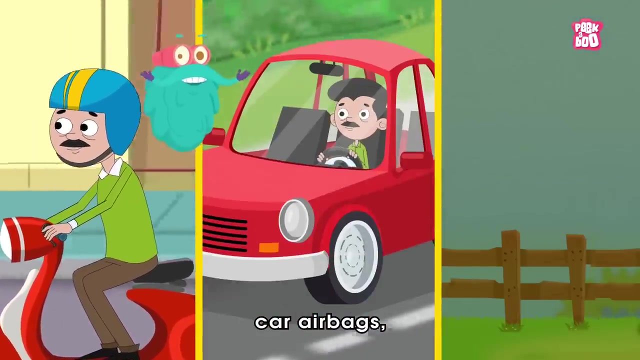 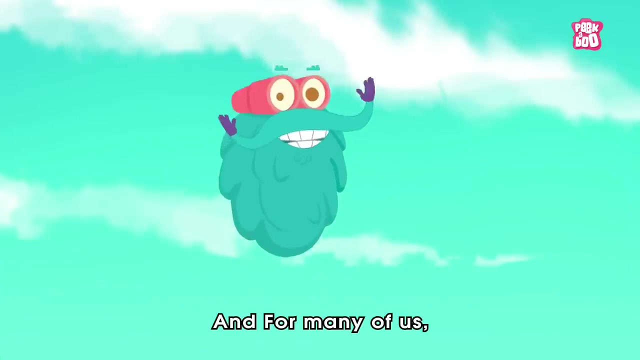 Yes, plastic revolutionized medicine with life-saving devices, made space travel possible, lightened cars and jets, saving fuel and pollution, and saved lives with helmets, car airbags and equipment for clean drinking water. And, for many of us, plastic has become integral to our daily lives. 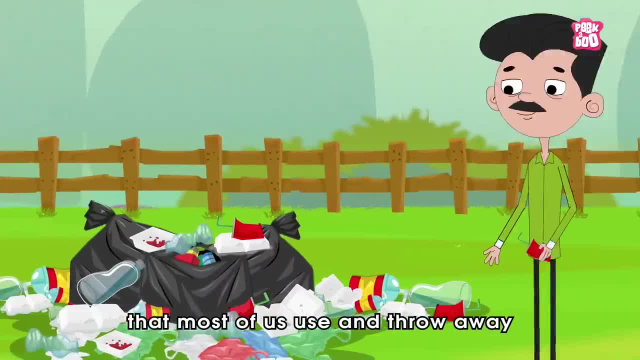 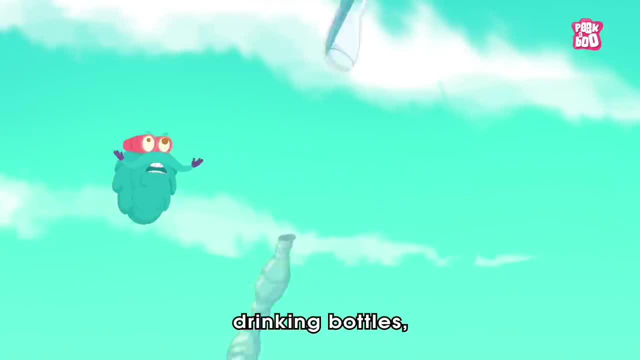 But the problem is that most of us use and throw away more plastic than we need: Things like grocery bags, drinking bottles, straws, food wrappers and plastic packaging around toys- This kind of plastic that's used only once before being thrown away. 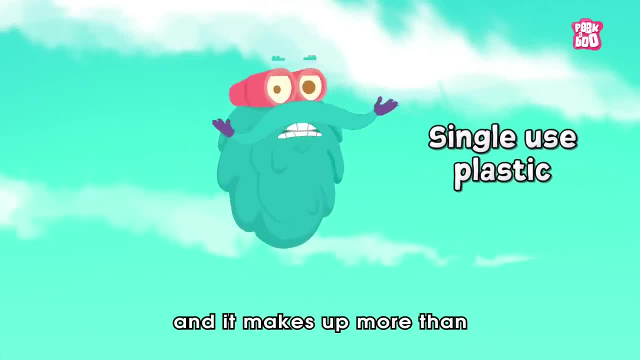 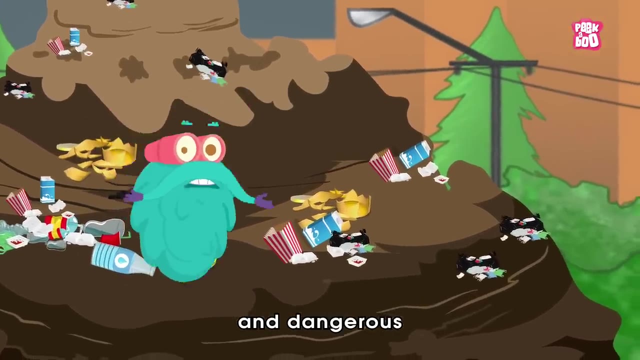 is called single-use plastic, And it makes up more than 40% of all plastic trash, And this short-lived use of millions of tons of plastic is quite simply unsustainable and dangerous for our planet as a whole. Now comes the most crucial question.